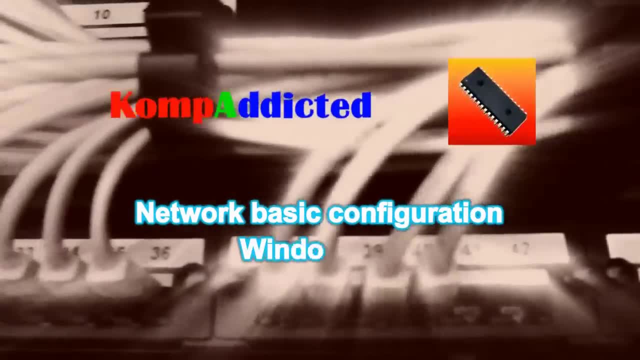 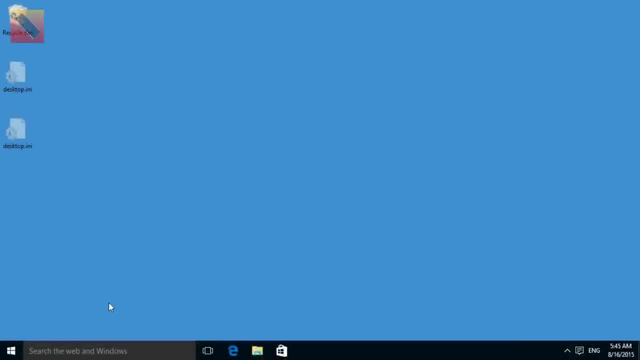 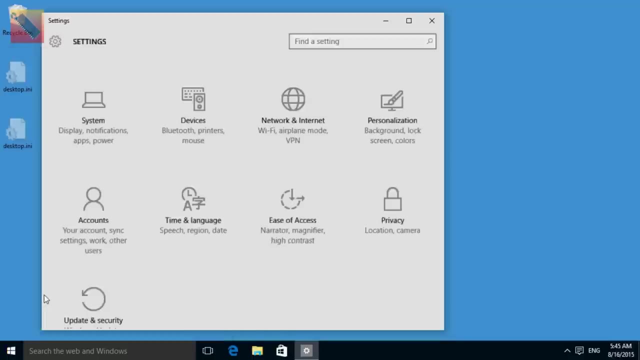 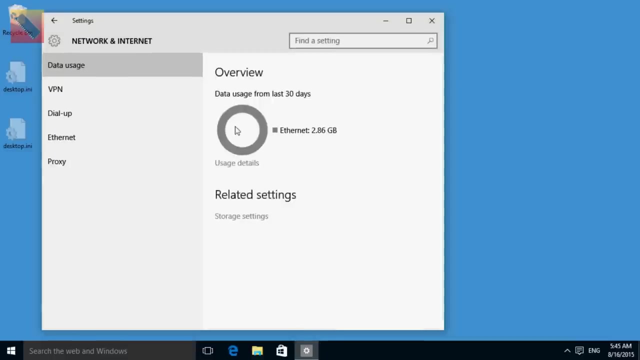 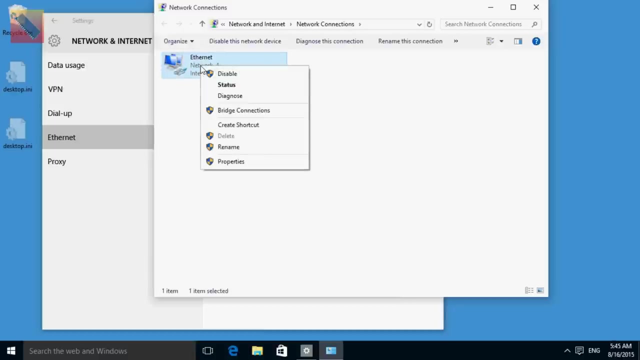 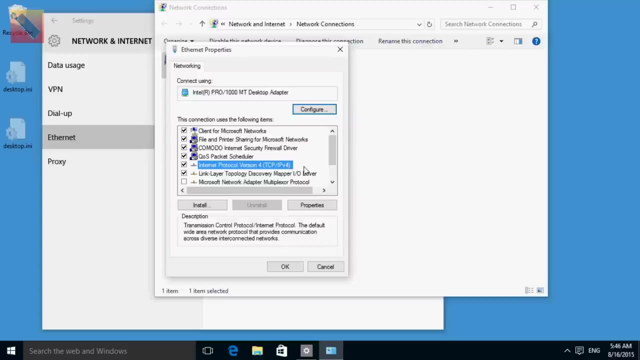 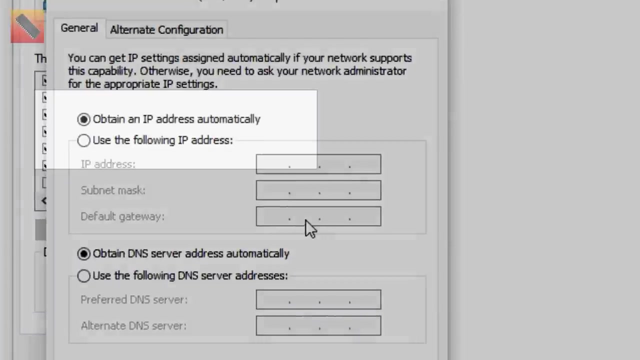 To get to the network configuration you have to select settings: network and internet ethernet. change adapter settings. Then right click to get local menu and select properties. Select internet protocol version 4.. Most frequently everything will be done automatically because the options obtain NIP address automatically. 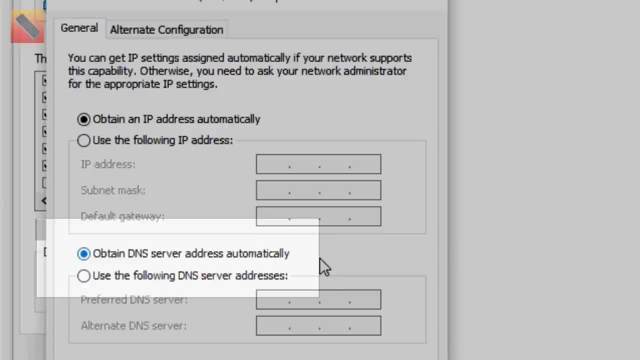 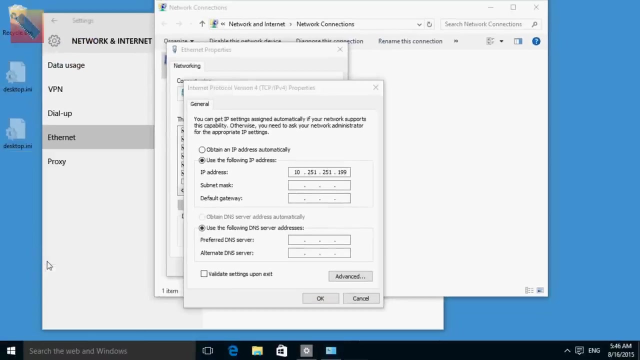 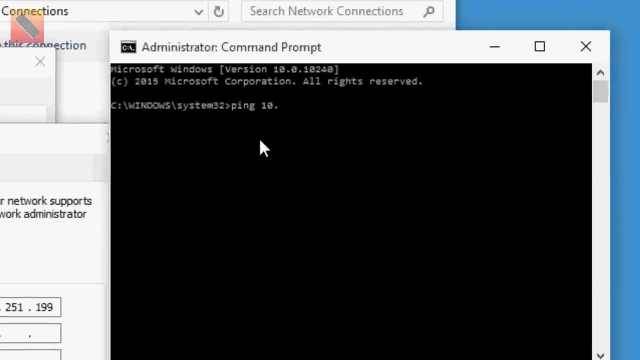 and obtain DNS server address automatically are selected, you don't have to write anything in the edit fields below. However, sometimes you will have to set the network configuration manually. First you enter the expected IP address of your computer. If you are not sure if it is already used, open the command line and ping to this address. 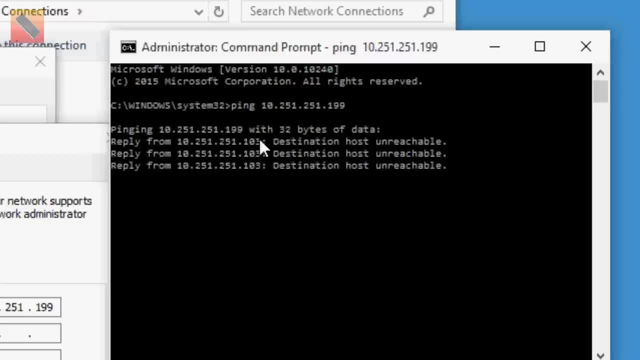 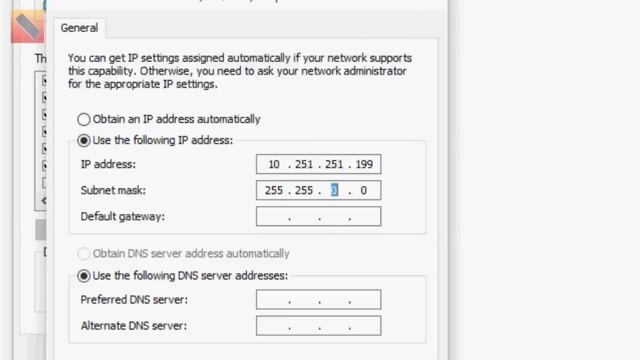 No answer, So we assume the address is OK. Next you have to give the subnet mask. Most commonly it consists of three numbers of 255 and one number of 0. You will enter the address of default gateway. It can be, for example, the address of your home router or modem. 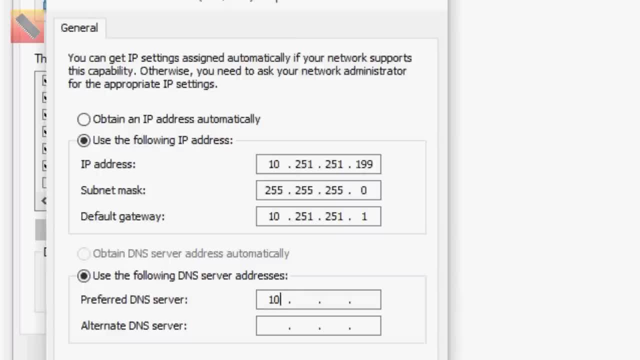 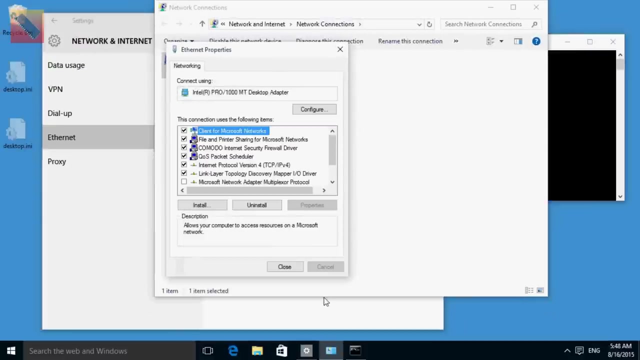 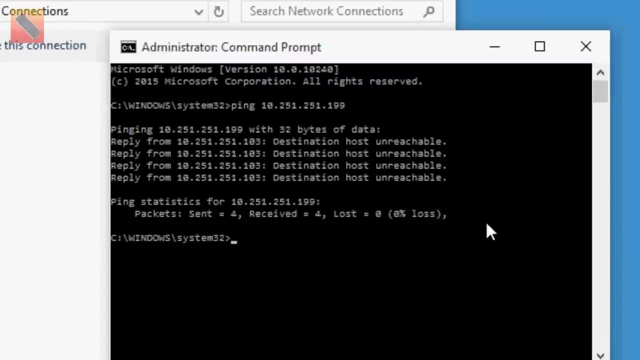 The first DNS server can be also the address of your home modem. You can also use the address of google DNS server, four numbers of 8.. Let's save the configuration. Now let's ping to googlecom to check if it works, OK. 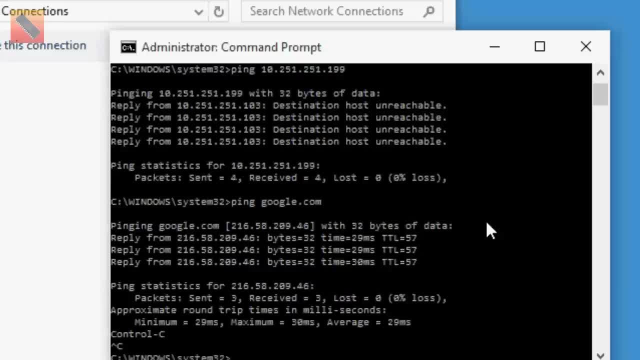 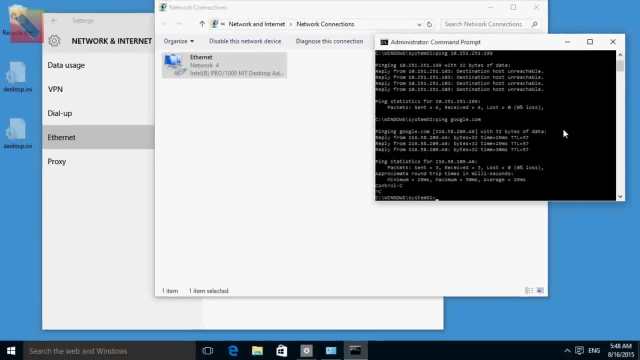 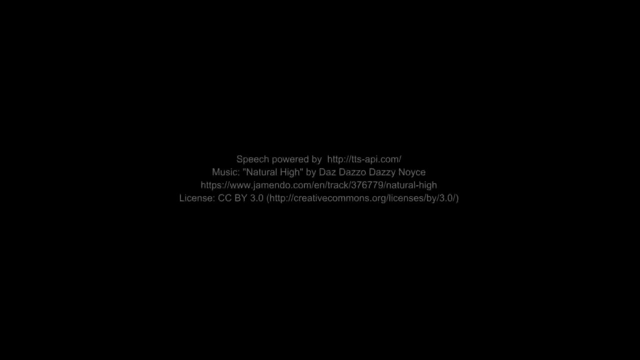 Looks everything is OK. If there were no answer, you should check the configuration again to find the problem. The reason could be wrong address of the default gateway or the DNS server. 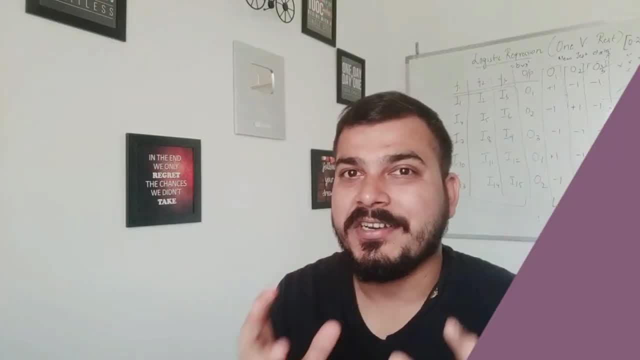 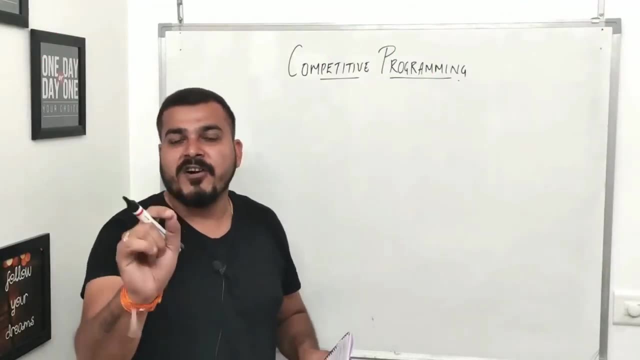 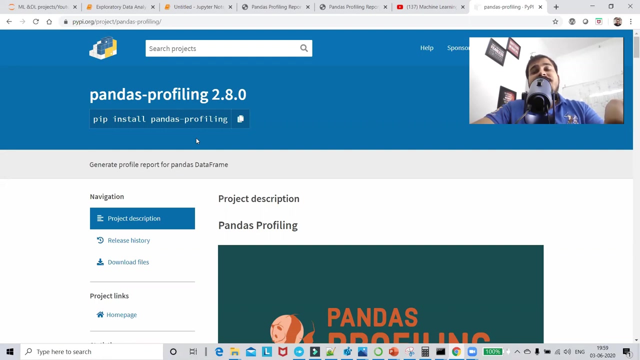 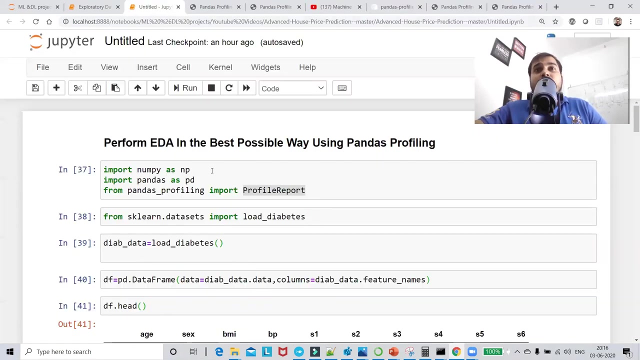 Hello, all my name is Krishnayak and welcome to my YouTube channel. guys, Today, in this particular video, I am going to discuss about how you can actually do exploratory data analysis. Now, before going ahead with respect to this particular video, guys, if you are looking, 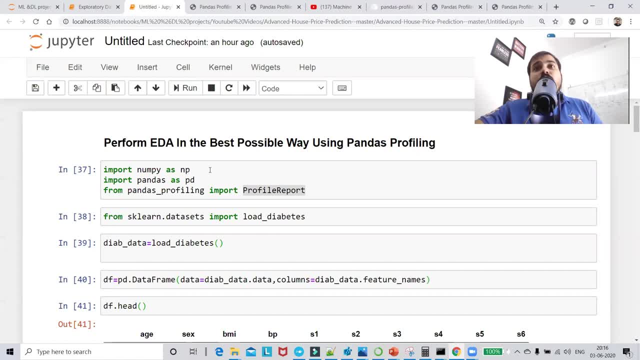 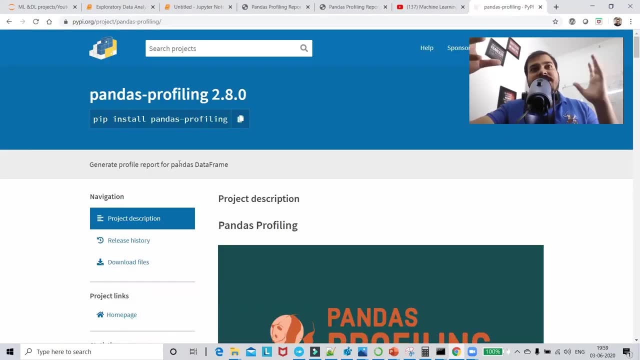 for career transition advice towards data science. please make sure that you watch this video till the end, because at the end of this particular video I am going to share some important information to you all. But just understand that what if you have a data set and you don't have to worry about anything as such? use just one kind of libraries, understand. 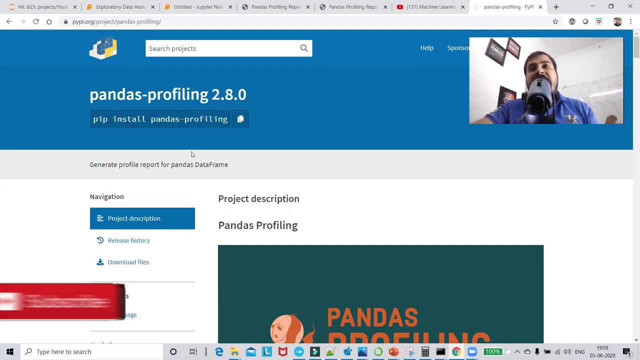 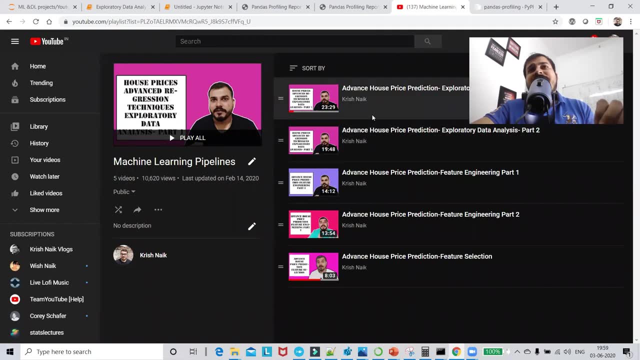 what all exploratory data analysis can be done on that right. Isn't it amazing? Because I will tell you why I am saying these specific things. You know, I had actually created something called as machine learning pipelines, and in this particular video, the first thing. 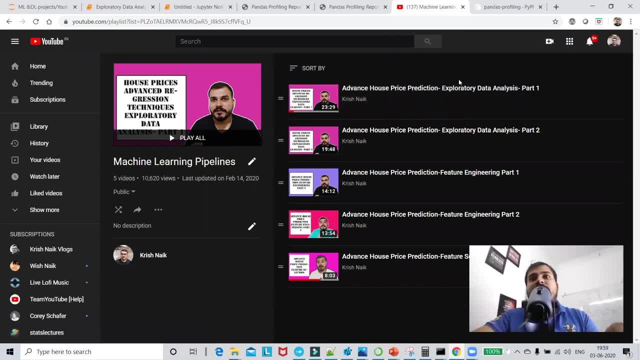 video was all about. if I just show you the video over here, the first video was about exploratory data analysis And in this video, when I was doing everything from scratch, it took me somewhere around 20 minutes to explain you all what all steps you can actually. 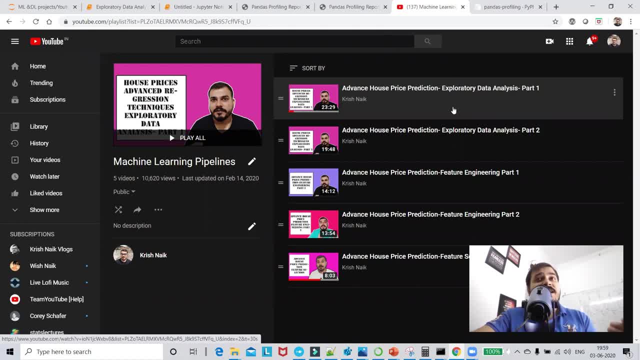 do. But what if? if I take the same data set, if I take other data set, you know I don't have to worry about, like, probably it may take somewhere around 20 minutes, but instead what I'll do is that I will just try to complete it within five minutes, you know, just by executing two.